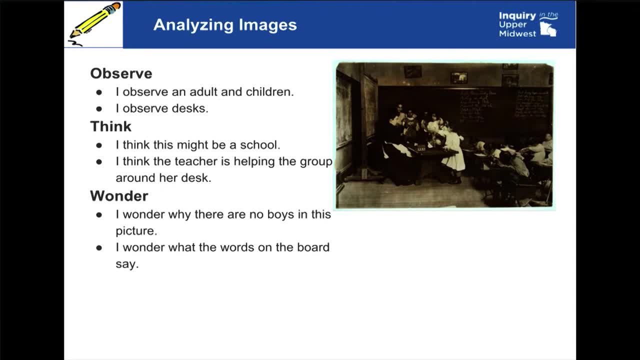 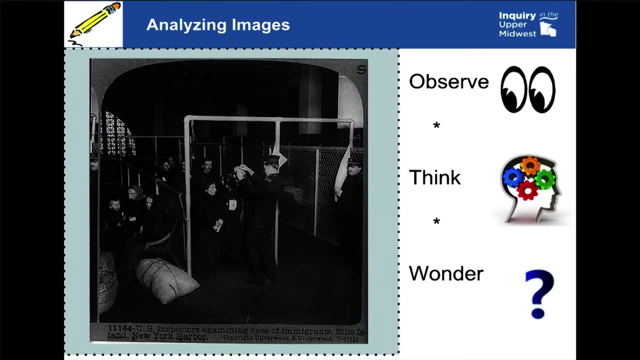 words on the board say: Observe, Think. Wonder is a really great tool for doing introductory analysis for images. So let's look at another one. So take a look at this image. What do you observe, What do you think, What do you wonder? 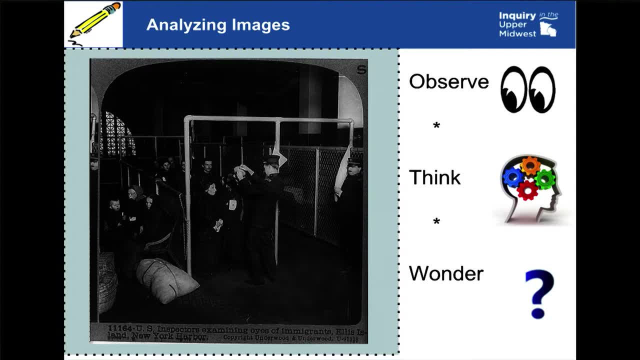 You might observe that there's a lot of people, that there's a person in uniform, that there are people sitting off to the side, You might think. are these people being examined? You might think, is that Ellis Island that I see at the very bottom in the caption, And are 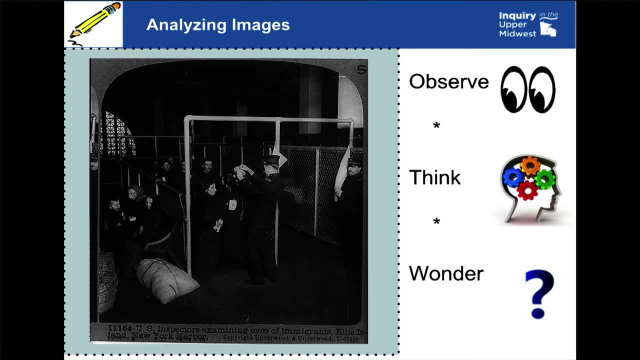 those people being examined coming into the country, And then you might wonder: Well, where are these people from and what are they being examined for? There's a whole lot of questions that can come from this, after you think about what you see and what you think. 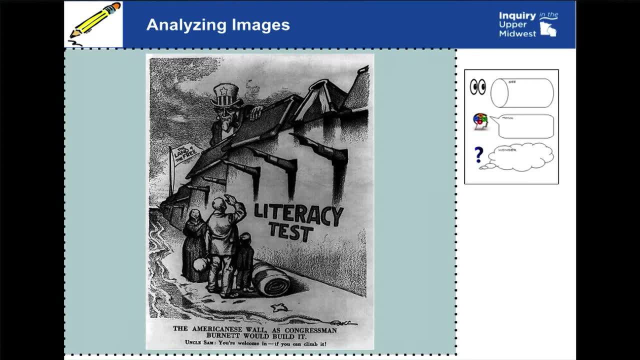 Let's take a look at another one. So political cartoons can be a little more complicated to analyze, but the Observe, Think Wonder tool can be a great way to get that introductory look at what is in this political cartoon. So what do you observe? 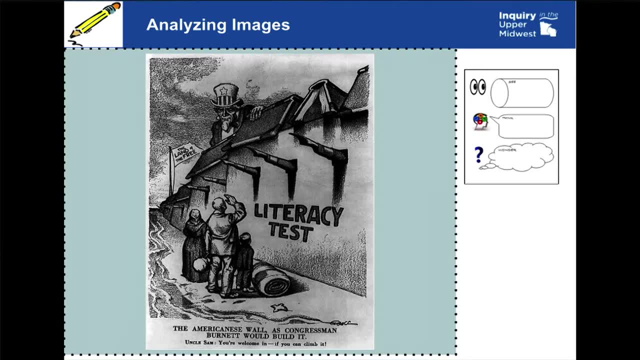 What do you think and what do you wonder? You might observe that there are three people standing looking up. You might observe that there is a wall with the words literacy test and books on top. You might think, I wonder. I think that those people might be immigrants. 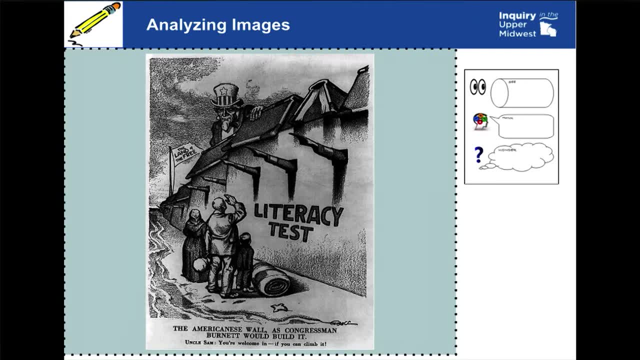 You might think that's Uncle Sam at the top And you might wonder where are these people from And what is the literacy test? There are a lot of great questions that can come from using the Observe Think Wonder tool and can bring great conversation into your classroom. 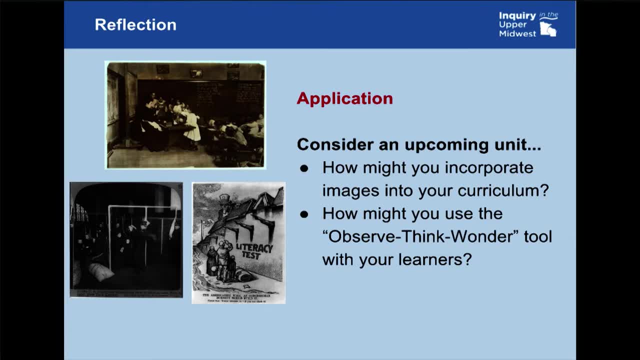 So now, how do you apply this in your class? So consider an upcoming unit. How might you incorporate images into your curriculum, Whether that's photographs or political cartoons or other types of images? So consider an upcoming unit. How might you incorporate images into your curriculum?